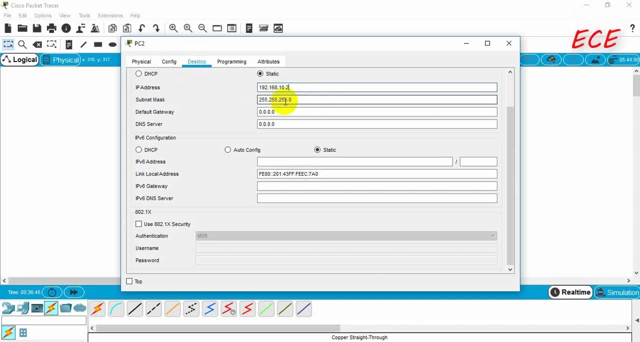 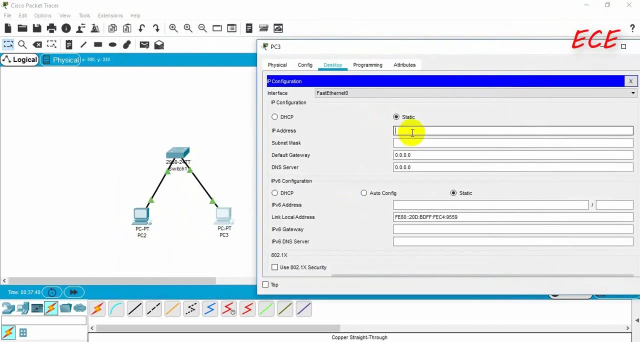 and if we press enter the subnet mask will be automatically added in this computer and then after this I will go to the next PC here, go to desktop, then IP configuration. here we will add IP address again and this will be the same IP address again. the net ID will be the same, but 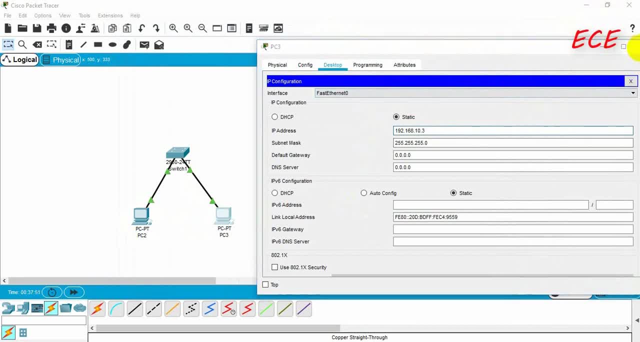 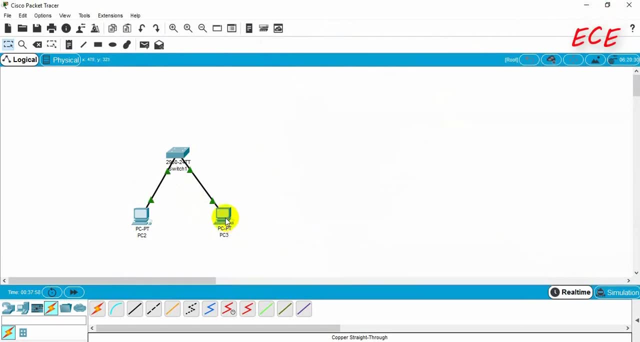 the host ID will be different. as this is our C class IP, you know that first 24-bit will be for net ID and the last 8-bit will be for host ID. Now you can see that the IP addresses has been updated here. now, if we you can see that the sign 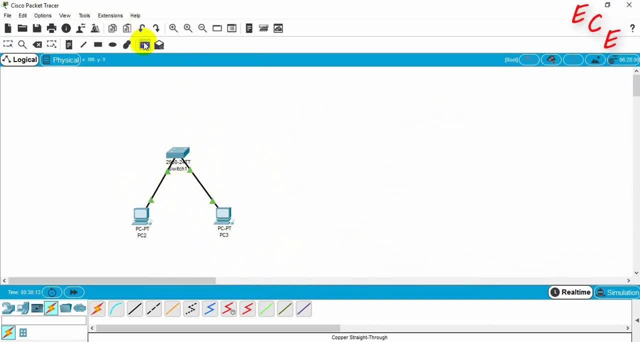 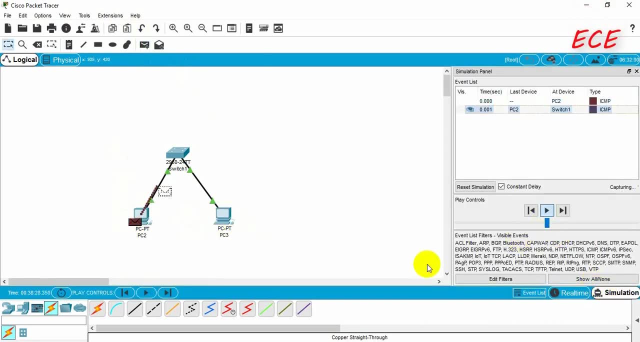 sign is also green, so we can send the data from here. now let's take a message and we want to send it from PC2 to PC3.. Now if we start the simulation, we can see the message is going to PC 3 from PC 2 and after sending that message it will. 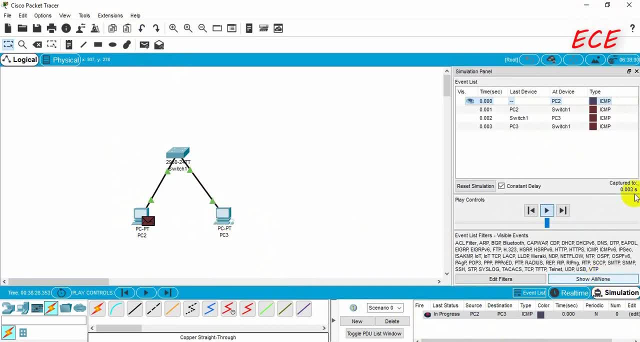 send back a signal to let the PC to know that the message has been sent successfully. let's see again. the message just reached PC 3. now PC 3 will send a signal back to PC 2 to let it know that it has received the message. then after that it: 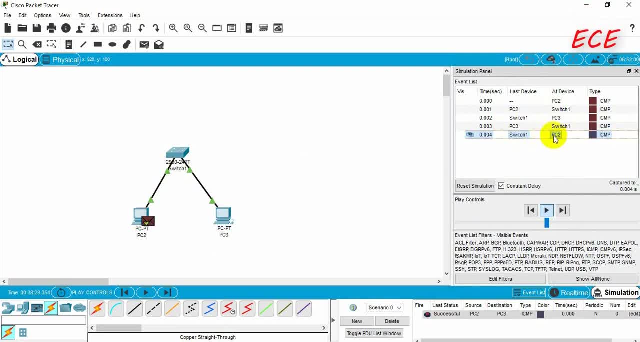 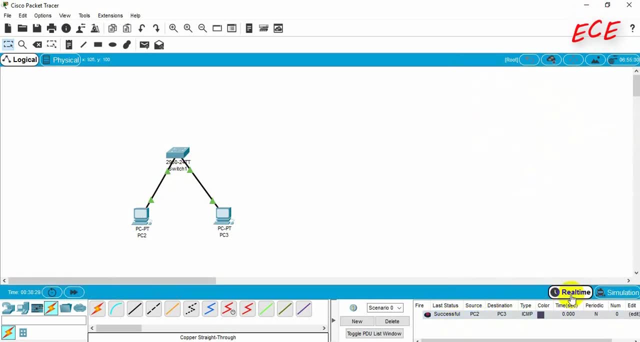 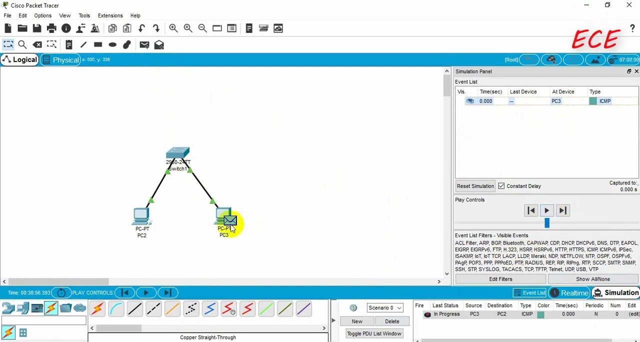 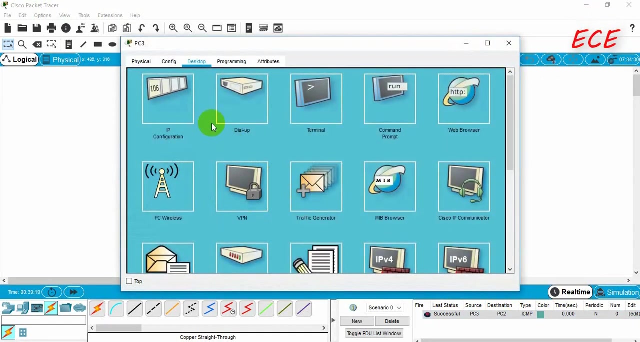 will be successful. now you can see that the last status is successful. source was PC 2 and destination was PC 3. let's send it from PC 3 to PC 2. now you can see it is also successful. now, if we change the IP address of this PC, we will change the network ID. that 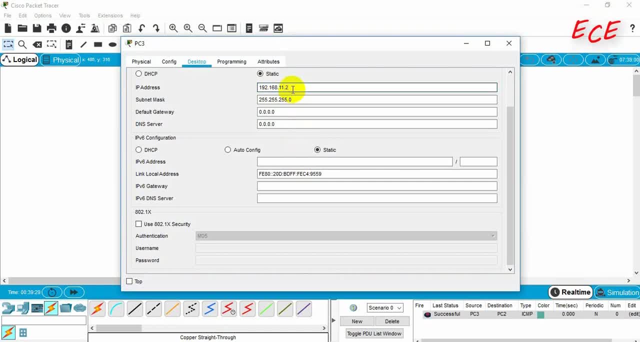 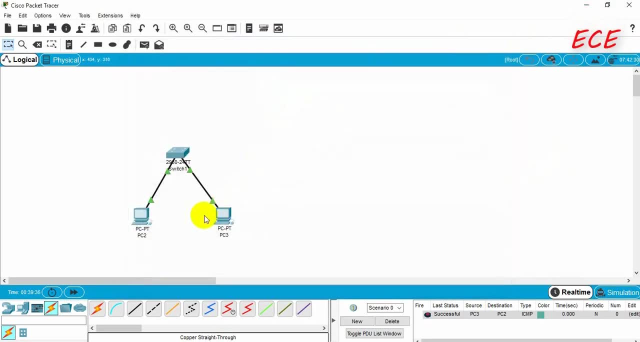 will be 11. so they, these two computer, are from two different IP address, two different network. now if we want to send message between them using a switch, we cannot send the message. you will see that the IP address is different from the other PC. now if we go to PC 3 and let's see that PC 3 has received the message from PC 2 to PC 2, 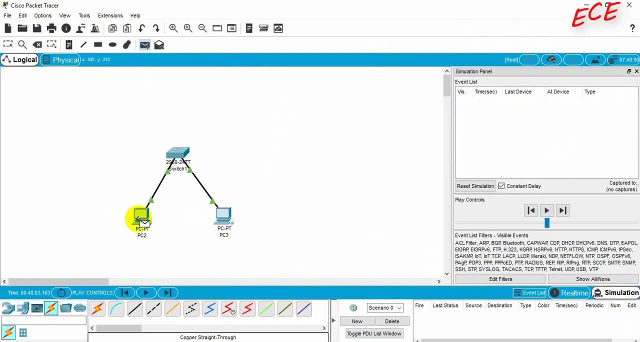 now, if we go to PC 3 and let's see that PC 3 has received the message from PC 2 to PC 2, go to simulation and if we send a message, you will see that it will not go. you can see the cross mark there and if we start the simulation, you will see. 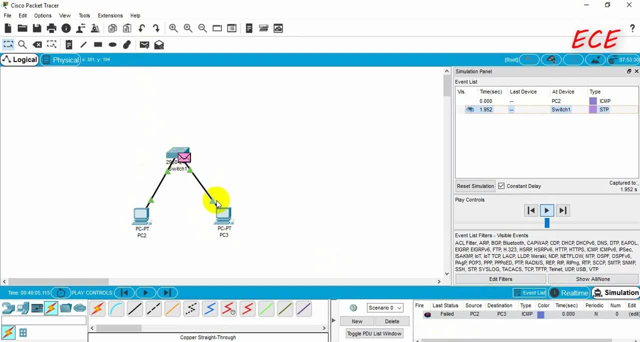 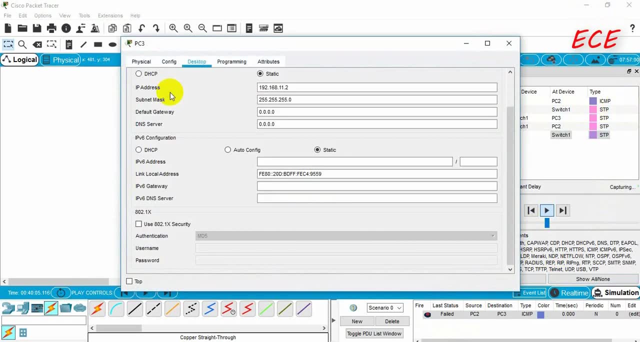 failed here. the message is not going because the two PC's in two different network now, as they have two different IP address. we cannot communicate with a switch if the IP address is different. so let's make it the same IP address again. only the host ID will be different and if we send the message, you can see. 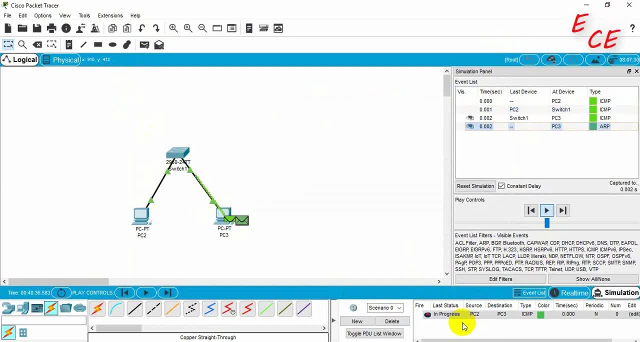 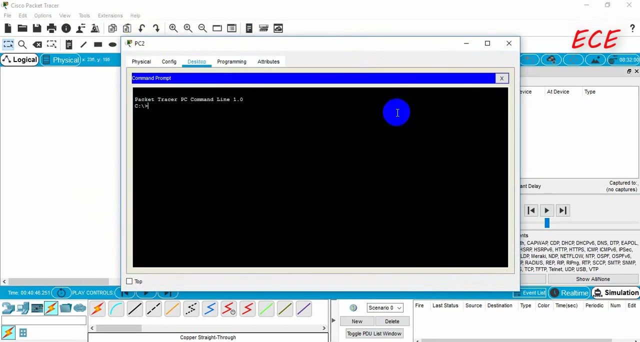 that it will be a successful process. after sending the message, it will send back a signal: you, you again, now you can see that it is successful process, and you, if we go to common prong, and here if we ping the PC3 from PC2, So we need to write PC3. 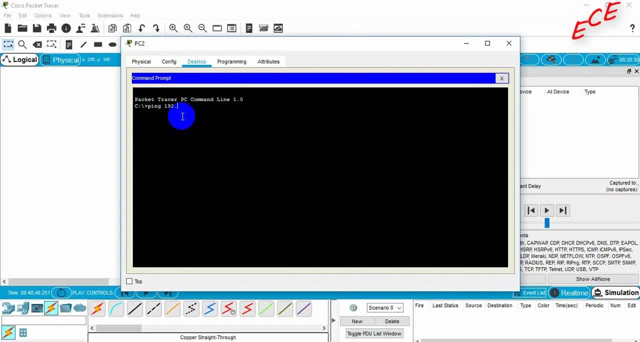 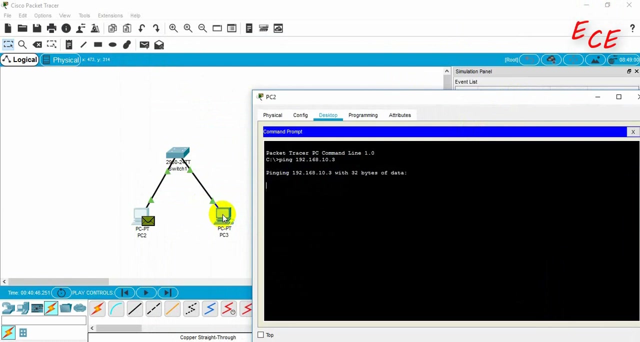 and if we are writing our PC2 then we need to do the same process. is ip address here: 192.168.11? sorry, dot 10.3. now, if we wait for some time, that pc will respond back. it can take some time. we can also ping from this pc too.